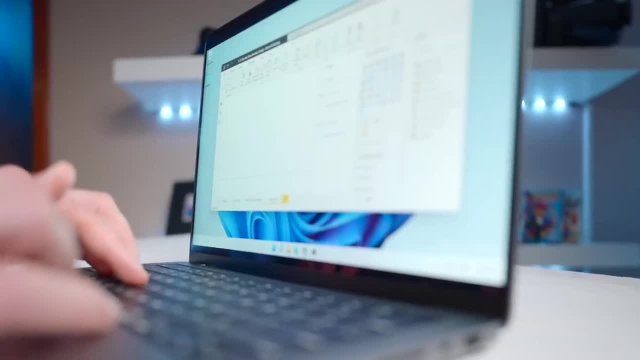 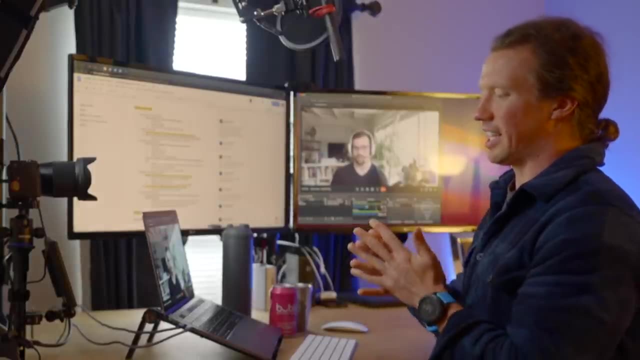 skills of a data analyst in order to continue to progress further in my job. This process has also been refined by my interactions from others that have not only gotten jobs as data analysts, but also hired others for these roles as well. My journey was filled with a lot of wasted time. 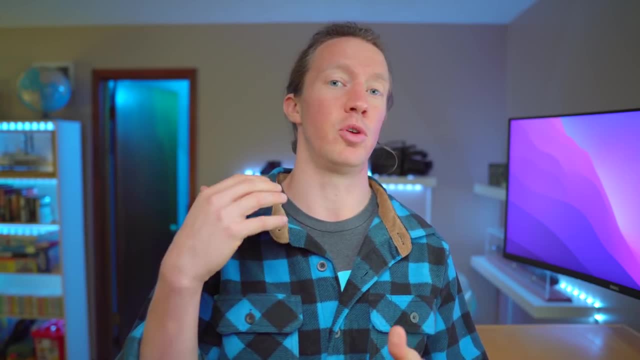 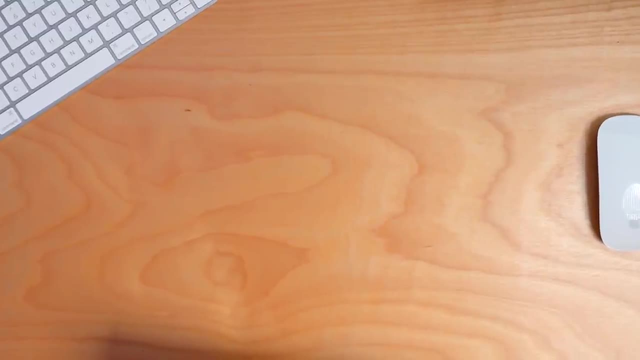 and effort, and so I'm hoping that this video helps save you effort and also time in learning the skills you need to know for your job. So let's break into my recipe for learning anything, and it's an iterative, two-step approach that I recommend taking. 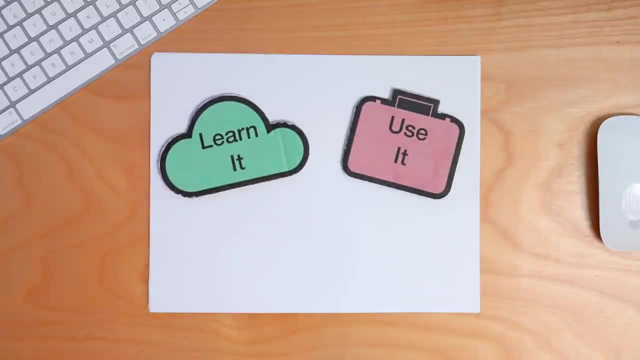 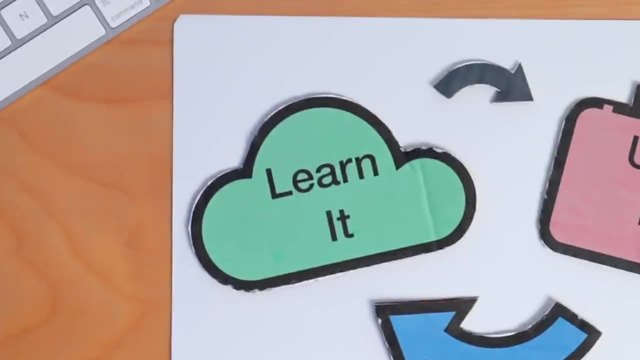 that can be used to learn more about data science. The process consists of learning it and then using it, So let's expand further into what you should be learning as a data analyst, And I feel that there are four general areas that you should. 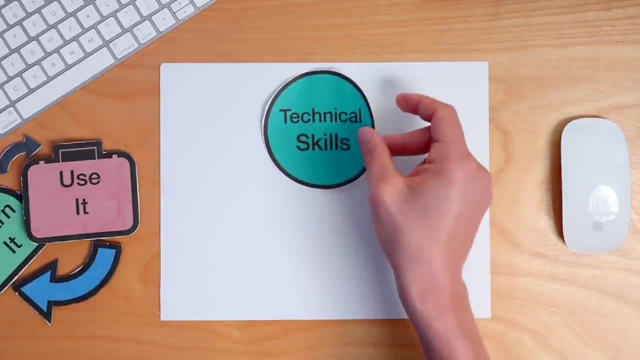 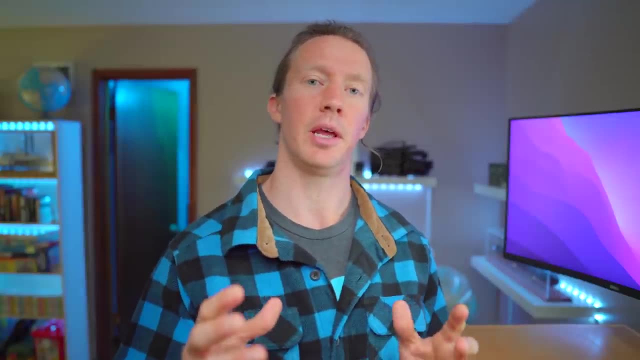 be focusing on that consist of technical skills, soft skills, analytical skills and domain knowledge. Don't worry, we'll go into all these general topic areas in a bit, but we need to move to that next step of actually applying it immediately after learning it and using it. 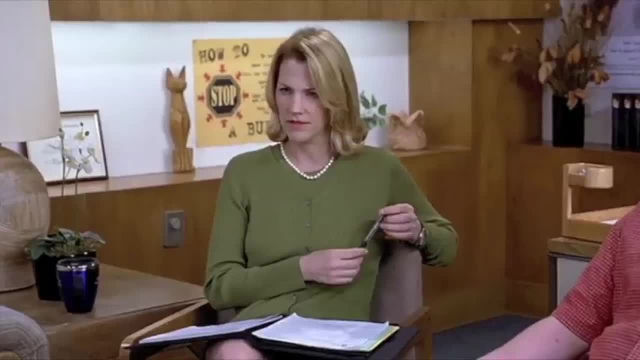 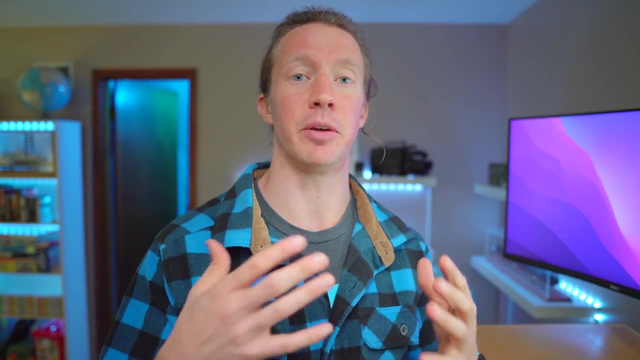 Is it true that if you don't use it, you can't learn it, Which in this case, is quite literally true, because the tools that I've learned in the past and haven't applied, I haven't been able to retain them. So I feel like this is a really key important. 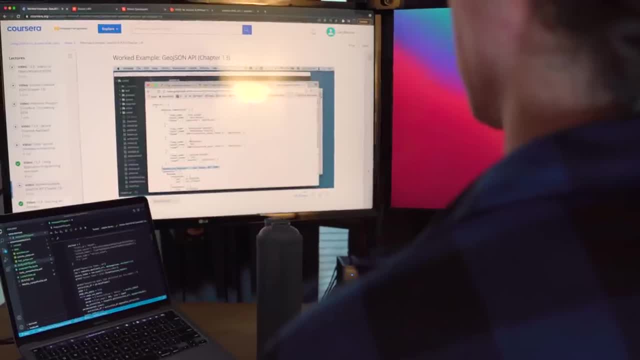 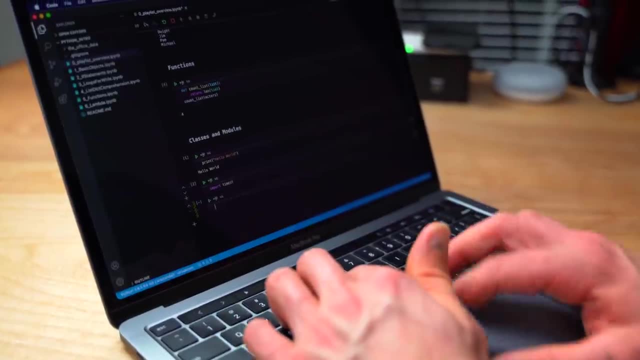 aspect in order to retain that skill. And you can use these skills in a variety of different ways, such as coursework projects on Coursera, portfolio projects for your resume, work projects for your job, and then also through teaching others. Now there's an added benefit of this second step. 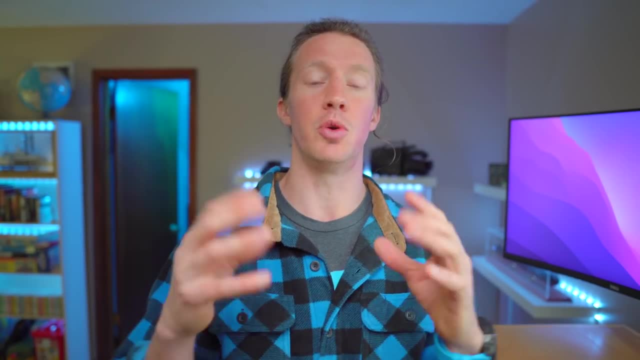 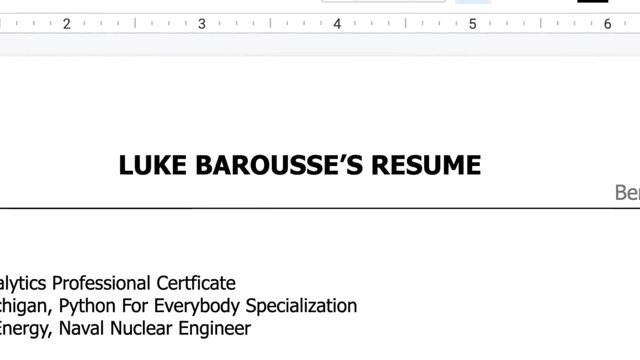 and that's that, because you're learning something new. you're learning something new and you're creating something with your new skills. you now have something to showcase to an employer as experience, So when you're searching for a job, you can now display this item that you created. 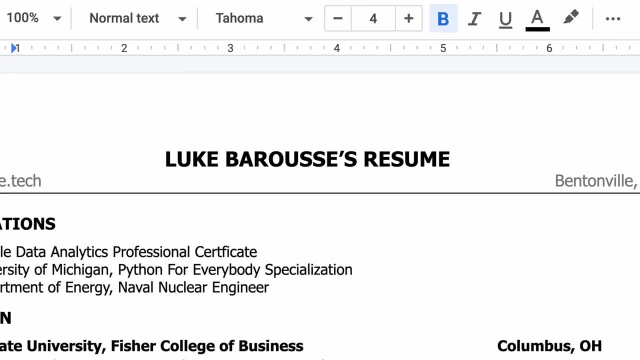 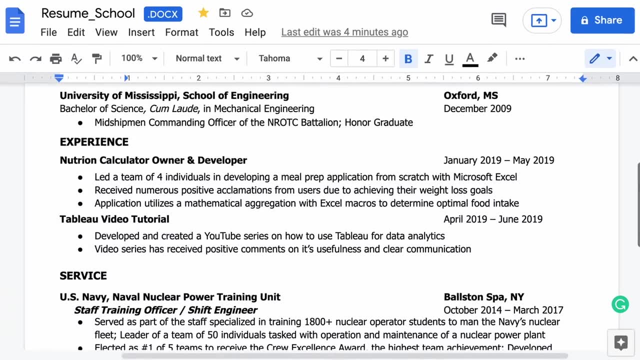 for employers to see. I've rambled about this before, but I think that online courses and certificates are great for this first step in the process of learning things, But if you don't have experience to showcase on a resume on how you use these skills that you learned, an employer is not. 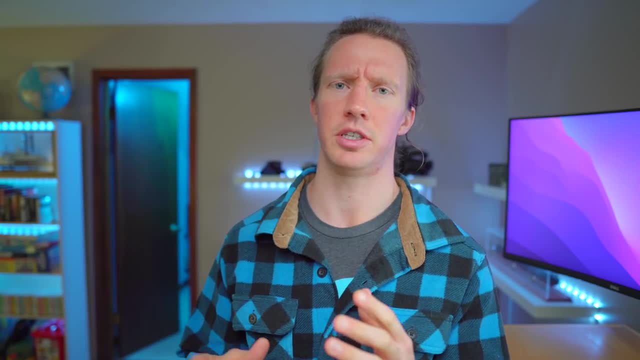 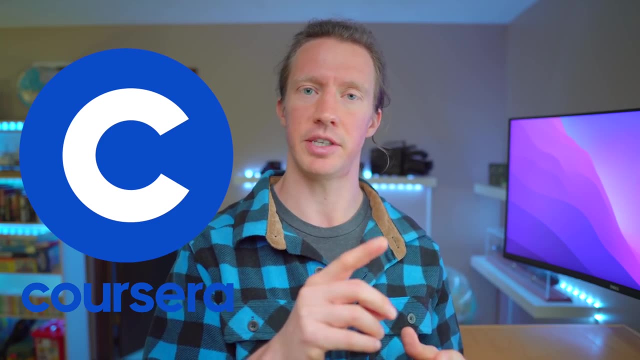 going to risk hiring you. And all of this relates directly to the sponsor of this video, Coursera. Coursera does a great job of hosting courses so that way you can learn the skills in that first step of the process, But also in that second step of using something. it then goes and 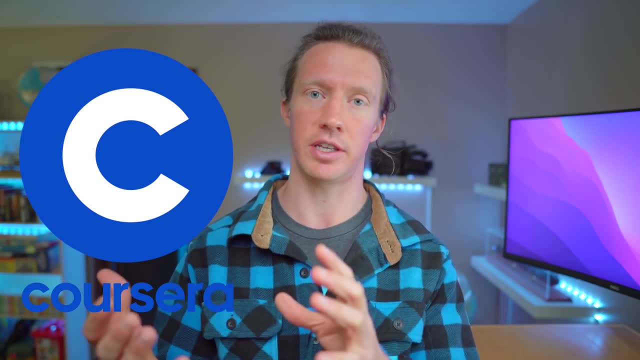 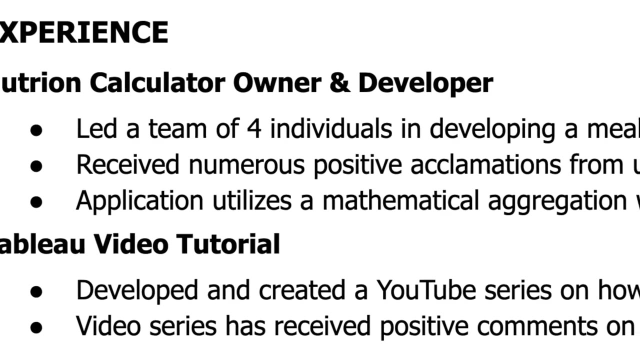 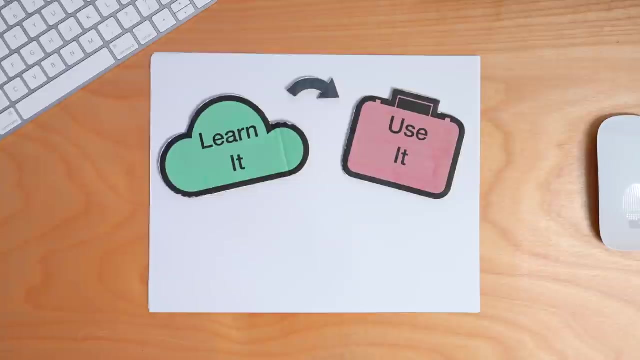 has projects available for its specializations and certificates, And this is great because you can not only display your certificate or specialization on a resume, you can also showcase those projects as experience for employers to see. So getting back to my learning process, So once you have learned a skill and then used it, it's then time to iterate back and 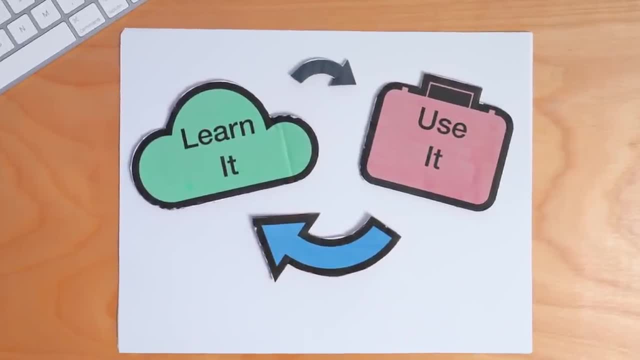 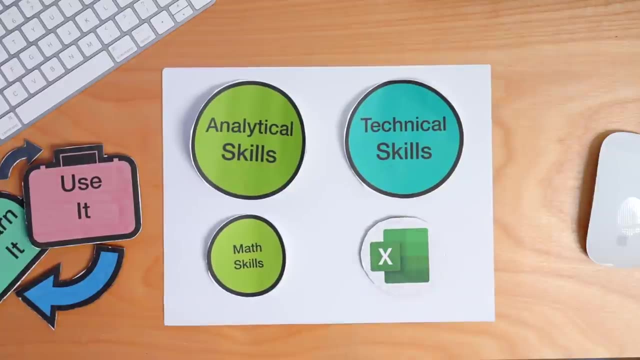 learn a new skill. So where do you actually start and what skill should you focus on first? for learning a skill, My preference is to start with those technical skills and then also incorporate those other skills, such as analytical or domain knowledge, while you're learning a. 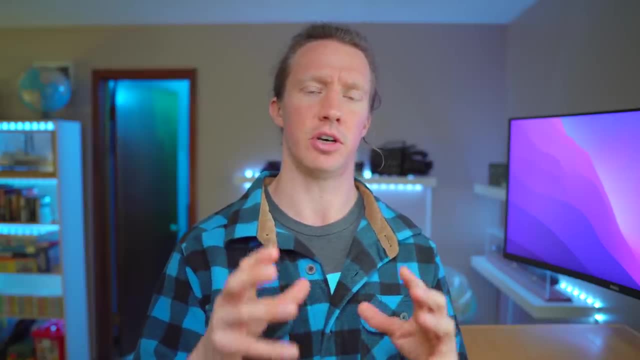 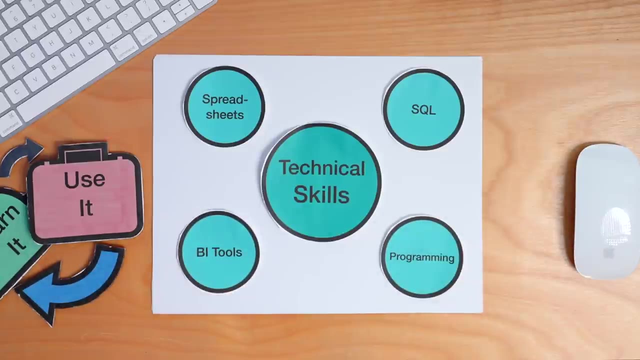 technical skill. So why do I say start on a technical skill first? So one? I feel like they're more tangible and they're easier to set goals that you can actually accomplish, Such as you can write out what functions you want to learn for Excel and then learn it. 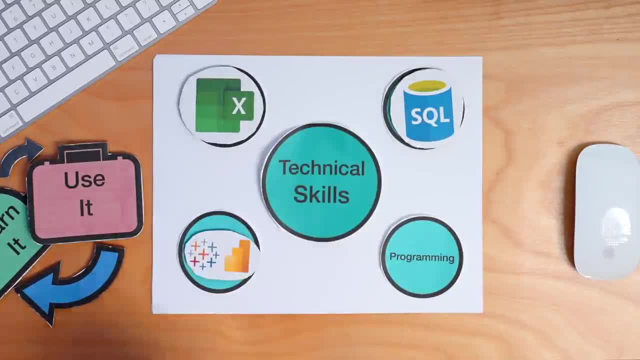 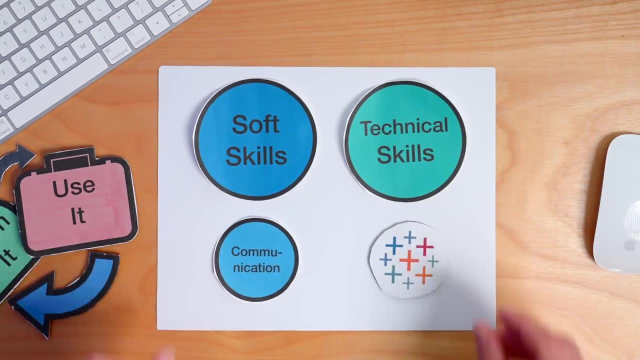 I also find that technical skills are funner to learn and I have higher motivation levels when actually setting out to accomplish that. And two, they allow you to apply other skills while actually focusing on that technical skill. For example, say, you're learning a technical skill. 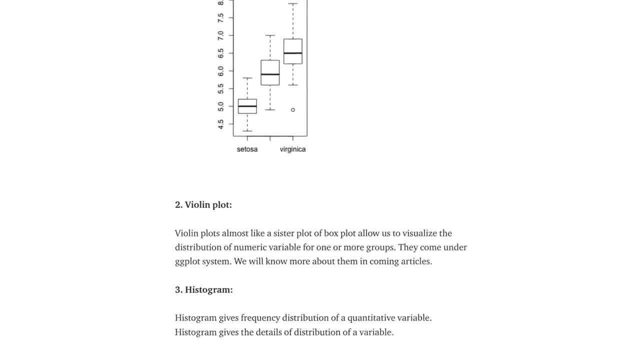 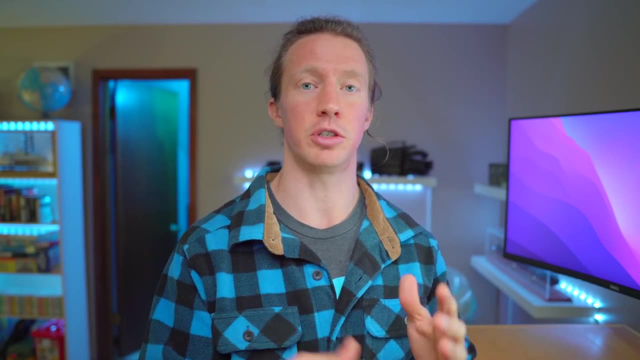 such as like R, you could also write a blog post about it, and this would showcase and build on your soft skill of writing. So, technically, you're not only focusing on technical skills, but you're also trying to incorporate those other skills as well. All right, so let's jump into my 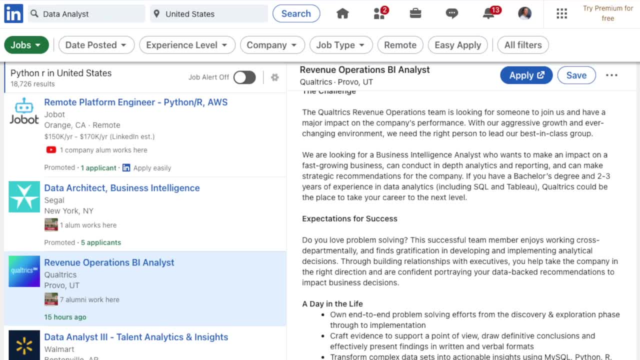 top five technical skills that I've learned over the years. So let's jump into my top five technical skills. So let's jump into my top five technical skill roadmap. So I recently did a data analytics project where I went through and scraped job posting data from LinkedIn. I was able to find 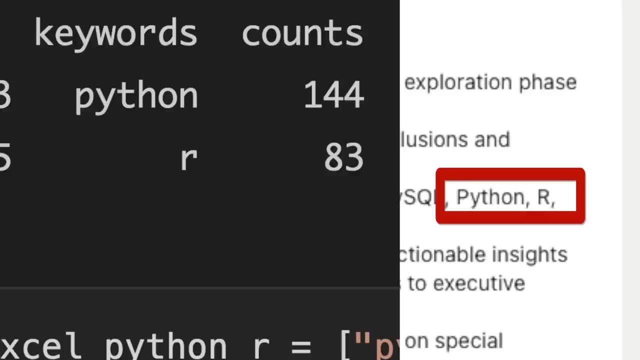 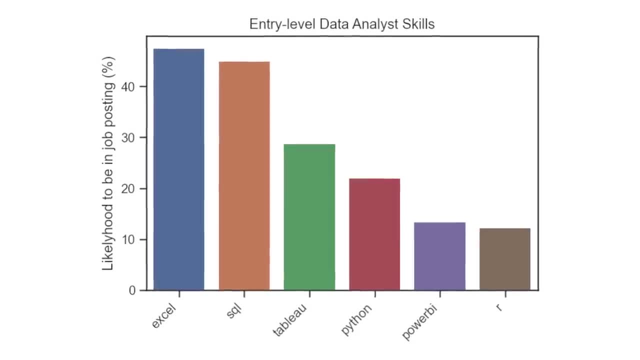 the most important skills for entry-level data analysts, based on how many times a skilled appeared in a job posting. So my insights from this project were this: that Excel and SQL are the most important skills to learn of a data analyst, as they comprise almost half of all job postings, Following in: 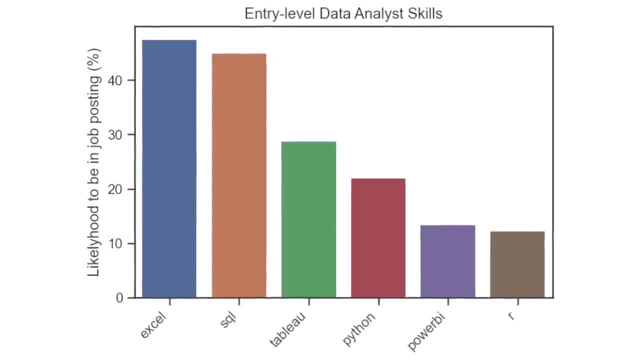 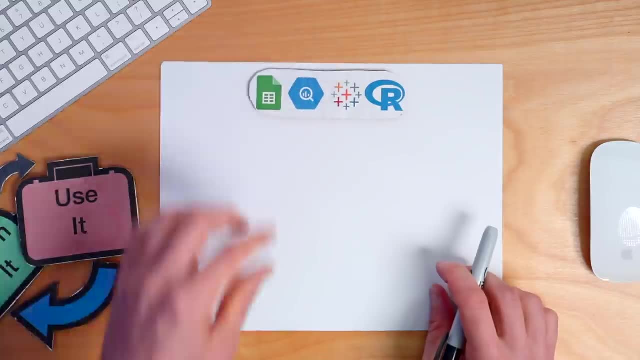 popularity are the BI tools of Tableau and Power BI, and then also the programming tools such as Python or R. So from this, my recommended roadmap is this: First, I recommend getting a brief overview of all the different tools. I think this is going to help with later on identifying tools that you 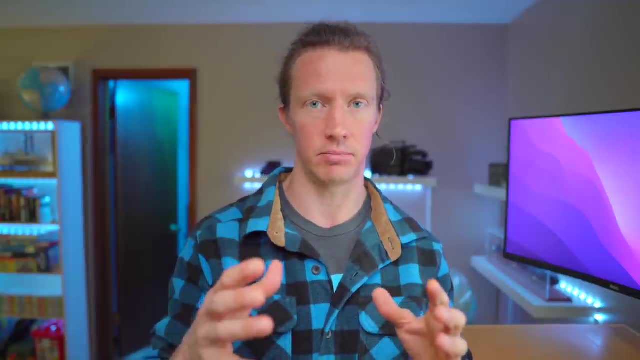 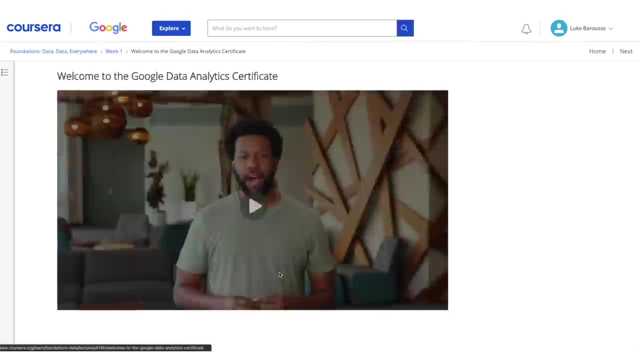 want to focus on, based on what your passion and interest is in. I like the Google data analytics certificate because it teaches you a lot about the popular tools of SQL spreadsheets, R and Tableau. And then, going back to my recommendation on how to learn, it not only teaches you. 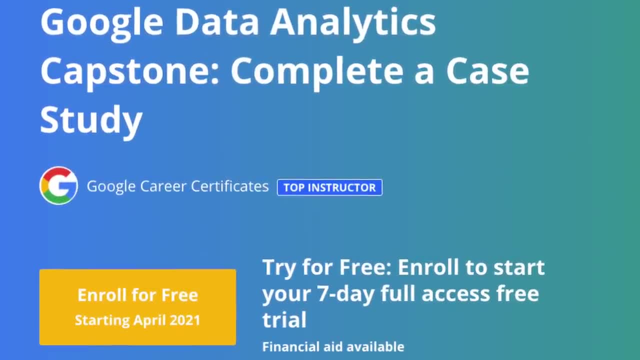 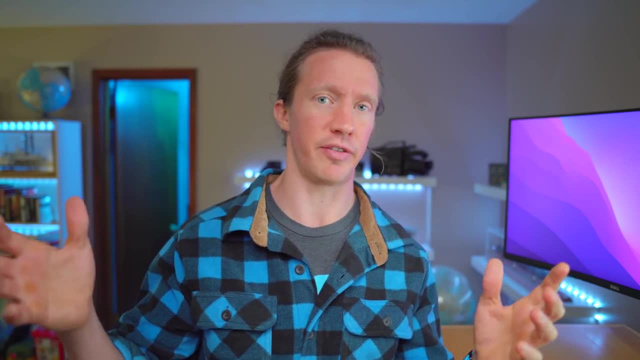 about these skills, but then you also implement these skills in a capstone project for the certificate. Now, this first step in the process is all about breadth, not depth, And the Google certificate is perfect for this, because you're not going to be a master. 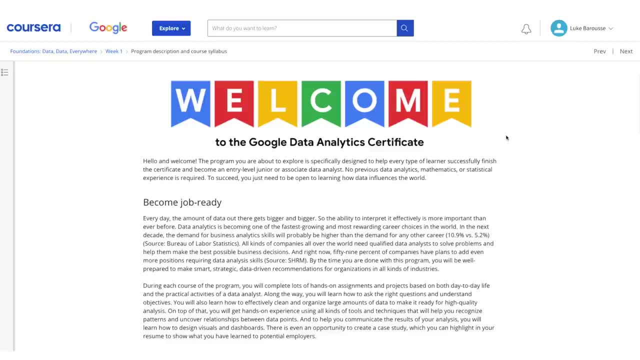 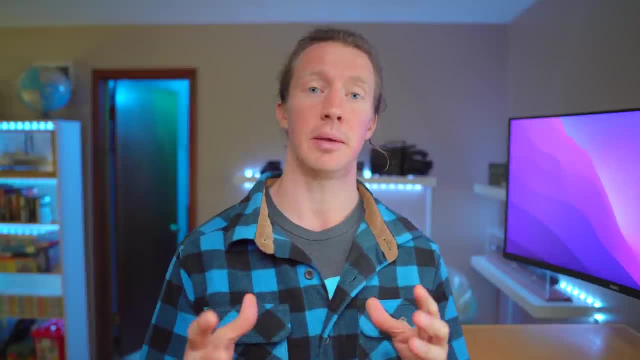 of any of these skills once you complete it, but you will have a general overview of these tools And you also have an introduction to other skills as well, such as soft skills and domain knowledge. Next, it's time to get into a mastering skill, And for this we need to focus on either Excel, 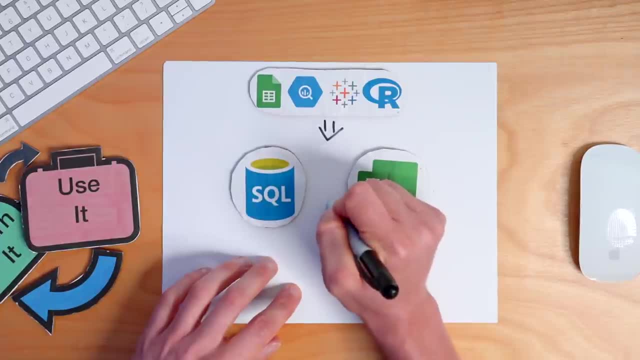 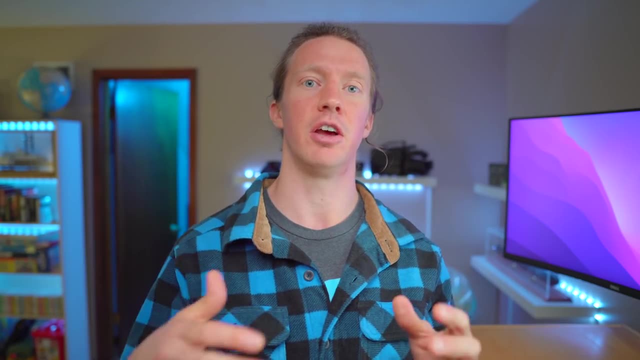 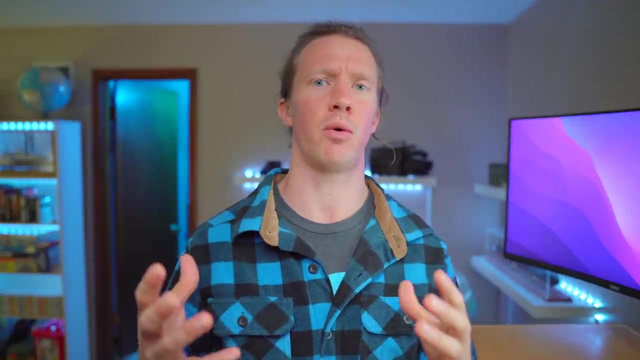 or SQL. I recommend these two most popular tool data analysts because, from a probabilistic standpoint, if you have these two skills, you're going to be able to learn a lot more about them. If you're looking for recommendations for resources to learn these types of skills, 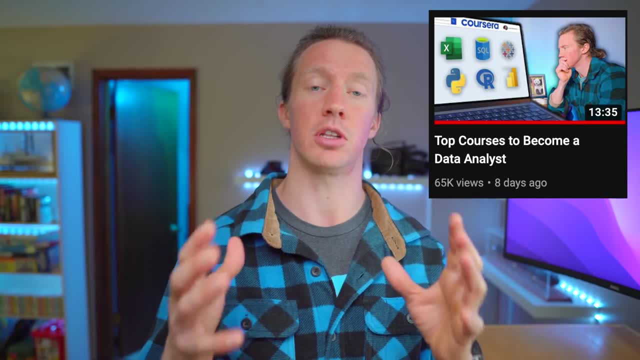 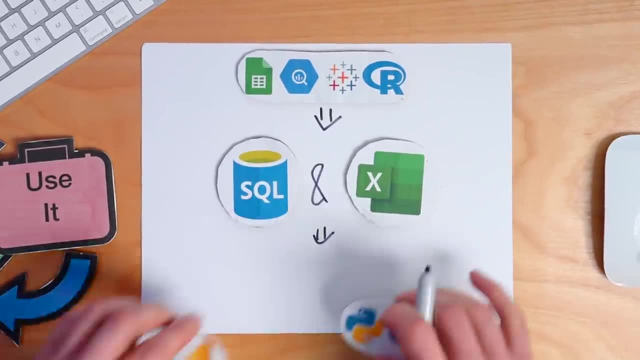 check out this recent video I did, where I went over some top courses to learn the skills of a data analyst. Next, after mastering both Excel and SQL, it's time to get into mastering other tools, such as BI tools and programming languages. Once again, when selecting one of these tools, 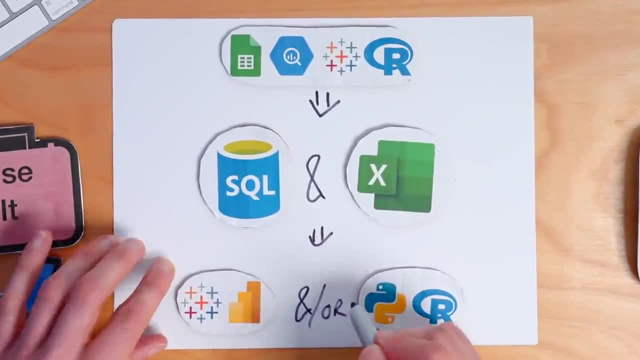 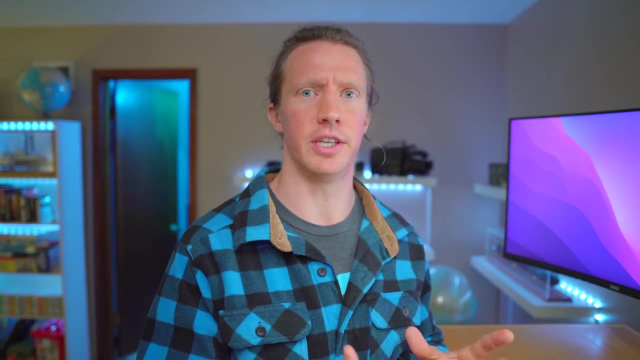 I'd go off what your passion is. Select one that you have an interest for and you really want to dive into and learn and apply other skills with. I think it's important to understand that you don't have to master every single one of these skills here in order to land your first job as a data analyst. My first job I landed with only 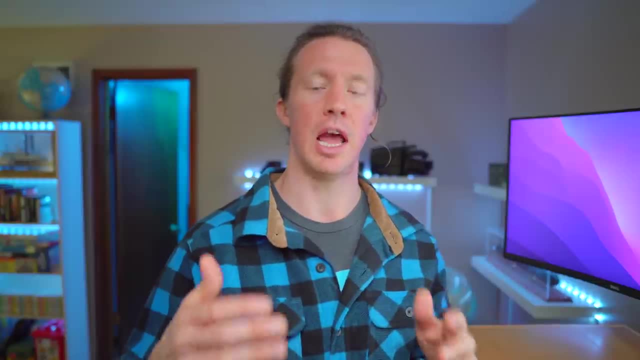 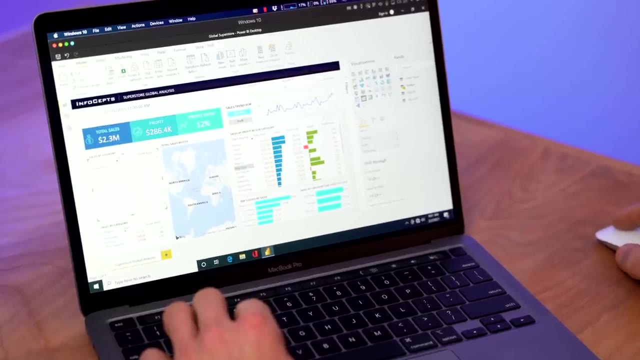 the skills of Excel, but I continued to progress my skills And because of that, I continue to advance in my career as a data analyst, being able to level up and get different opportunities based on the skills I was learning. So that's my roadmap for technical skills. But what about? 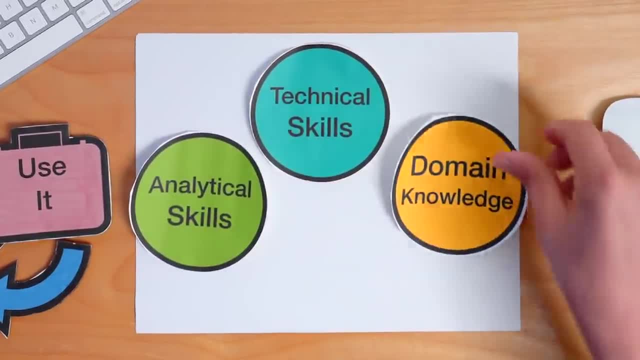 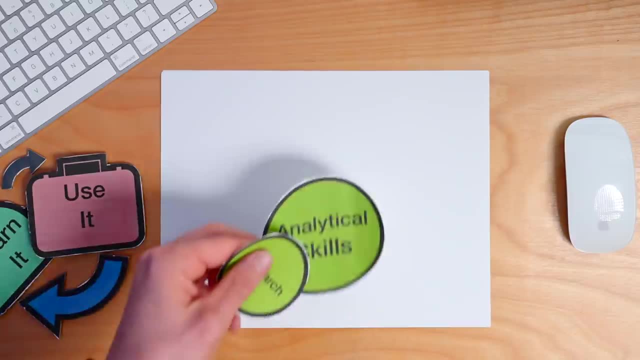 those other areas of analytical skills, domain knowledge and soft skills, And what do I mean by these skills And how do I incorporate them while learning those technical skills? Let's break it down. First up is analytical skills, And by this I mean things like problem solving, critical. 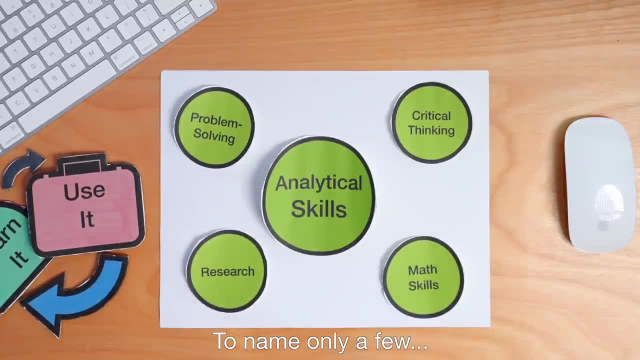 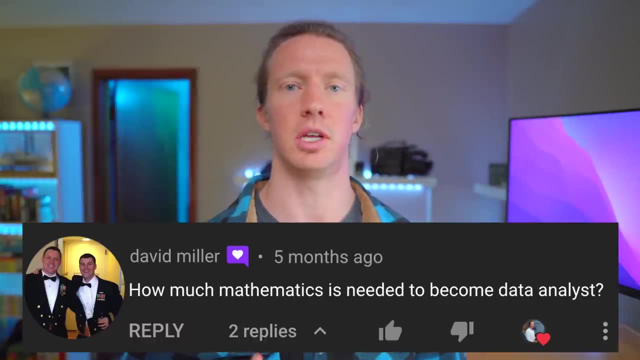 thinking, research and then math skills. So I get a lot of questions around this math skill- whether more in-depth training or studies is needed prior to taking any courses or prior to diving into the field of data analytics. Part of my life as a data analyst I was 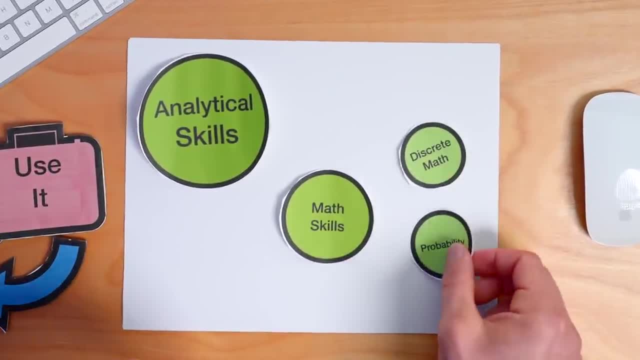 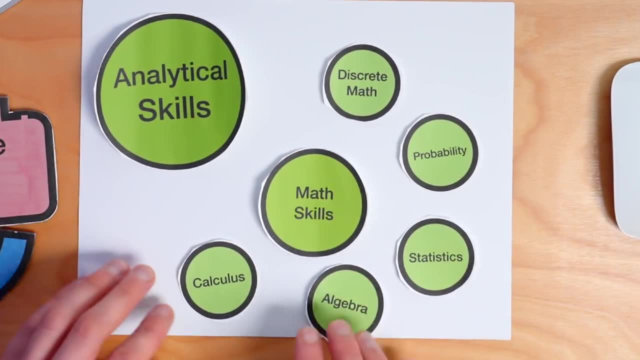 fortunate enough to be exposed to a lot of different math subjects, So everything from algebra to more advanced mathematics like calculus and differential equations. Because of this, and now being my role of data analyst, I can say that the most of the math that I've 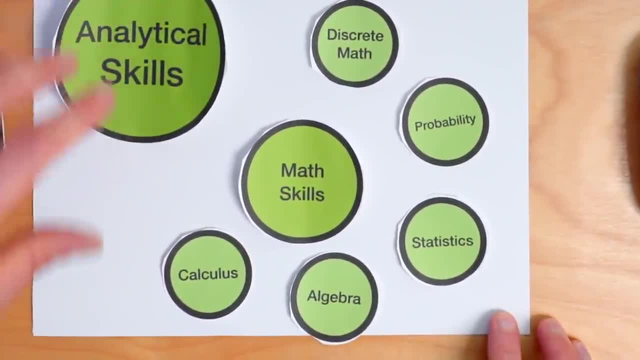 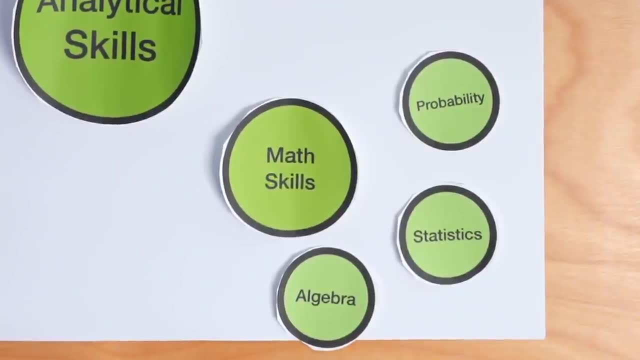 applied in my job has been pretty basic math and has focused on algebra, probability and statistics. I don't think subjects like calculus and discrete math are necessary, especially for entry-level data analyst roles, And so the good news is that for most secondary schools, 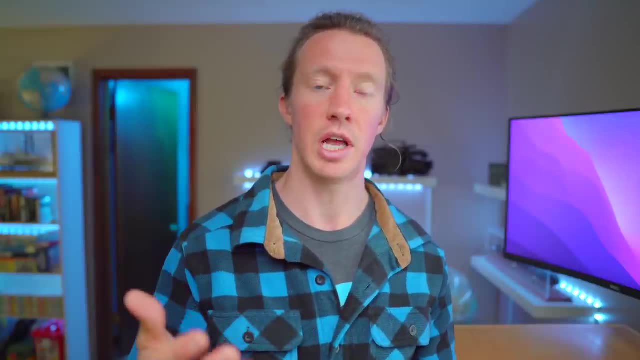 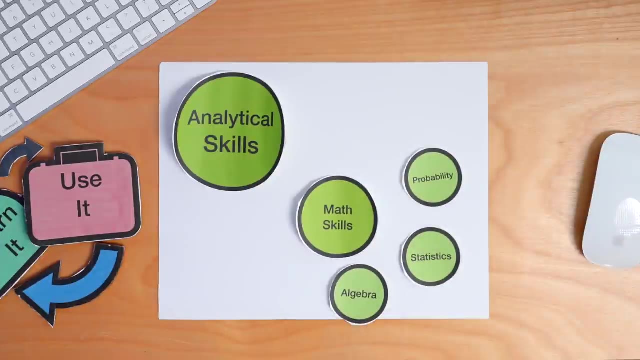 like high schools in the United States, you're exposed to subjects such as algebra and also other subjects like probability and statistics. So, based on this, I wouldn't necessarily worry that you don't have the math skills to get started. Instead, if you don't know something in 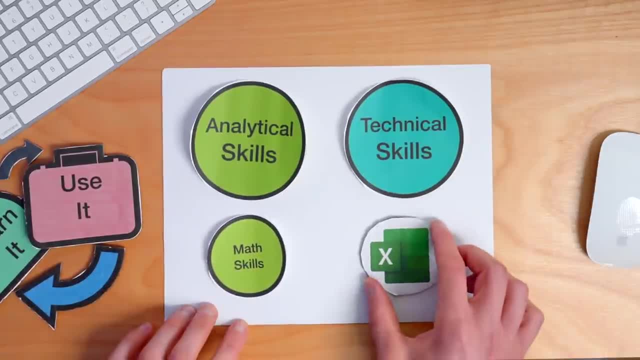 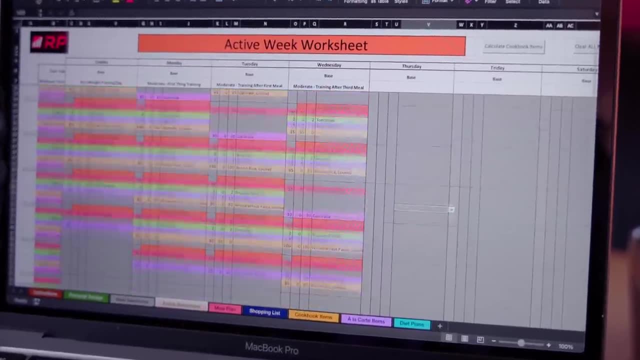 math. you can then learn it or apply it in a project as you're going along. So, getting back to how to apply analytical skills in a project, When I was learning Excel, one of my portfolio projects that I was working on in school was building a food nutrition calculator. This was 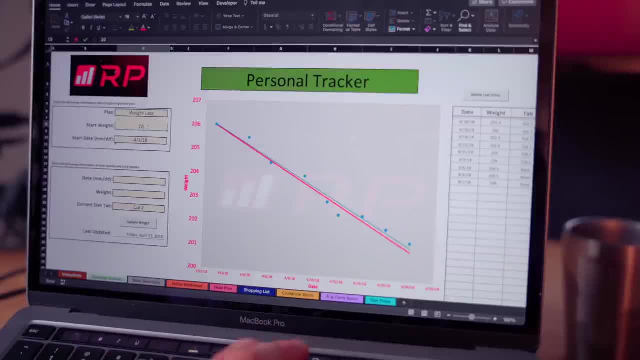 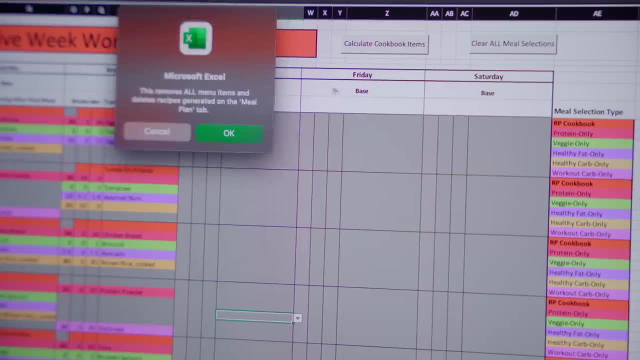 a spreadsheet that could tell you what to do and what not to do, And I was able to do a lot of it in order to be healthy. This project not only required learning Excel. it also applied probability and statistics in determining what foods to recommend, along with basic algebra in 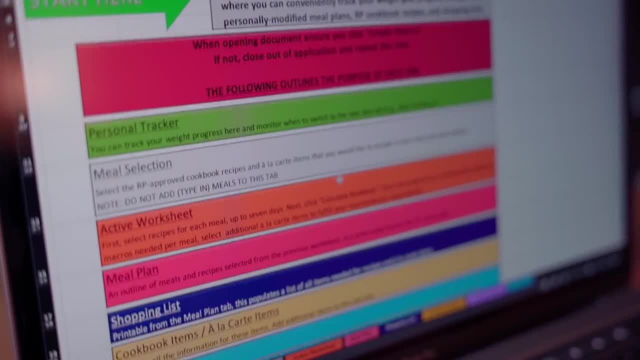 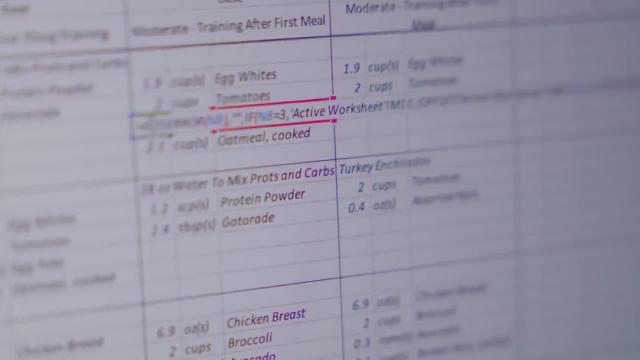 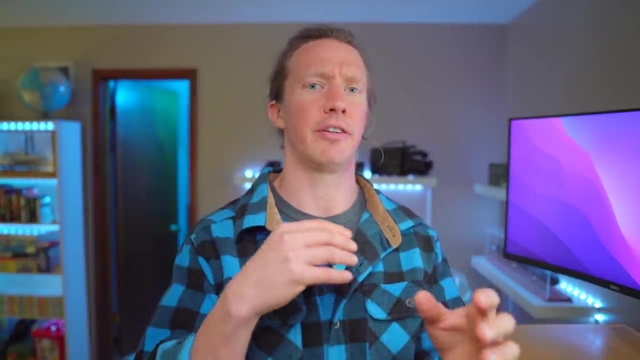 calculating macronutrient values of food. This project was not only great for teaching me the technical skill of Excel, but also testing my analytical skills in solving this problem of building this calculator. Interesting enough, this project got brought up multiple times in different job interviews I were in, specifically by interviewees that were interested in physical 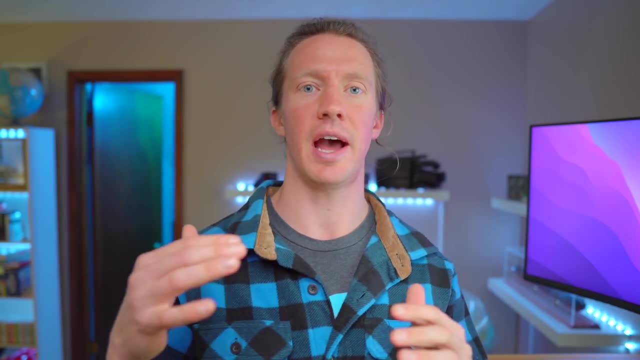 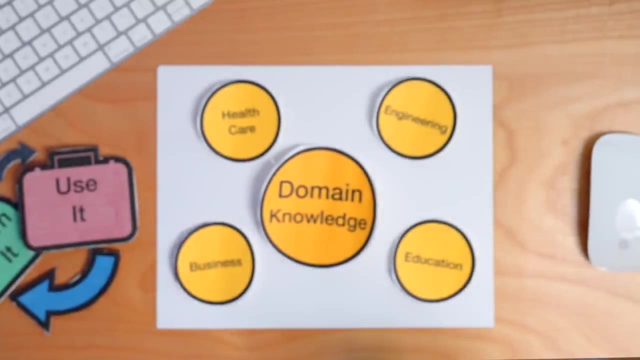 fitness and well-being, And it was really great because it allowed me to connect on a similar interest with the interviewee. Next up is domain knowledge, And this is knowledge of a specific discipline or field. So, for example, I recently asked you all what fields you were transitioning. 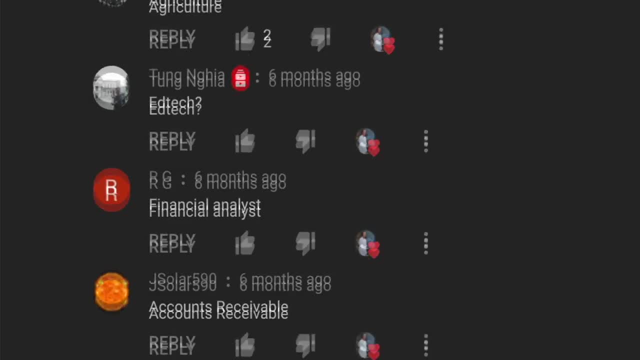 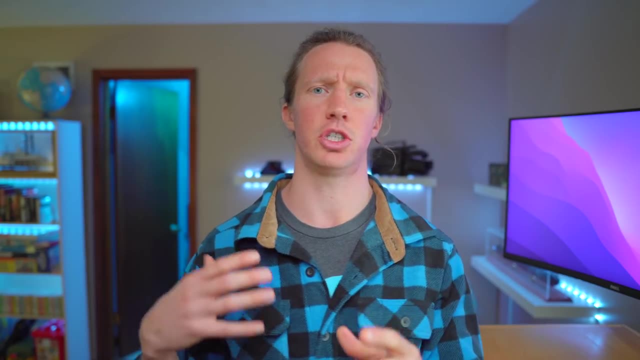 from to become a data analyst, And the results range from students in business and engineering to those working in an industry such as education and healthcare. From what I found, you don't have to actually switch industries or domains in order to become a data analyst. In fact, what I found, 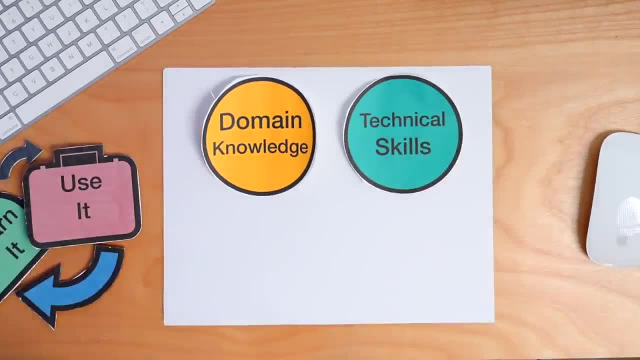 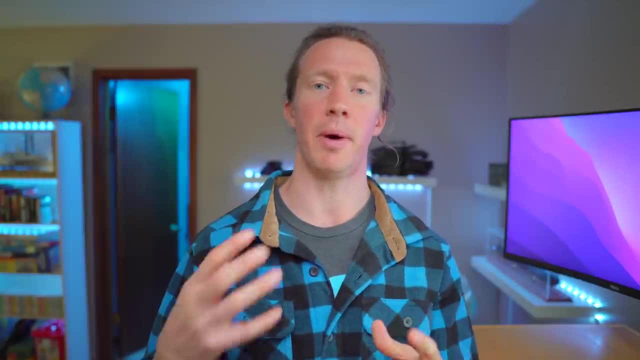 is those that have the most success in becoming data analysts, apply those newly learned data analytical skills in the current domain or industry that they're in. As an example of this, in my first role I was working in the procurement industry, working only with the skill of Excel. 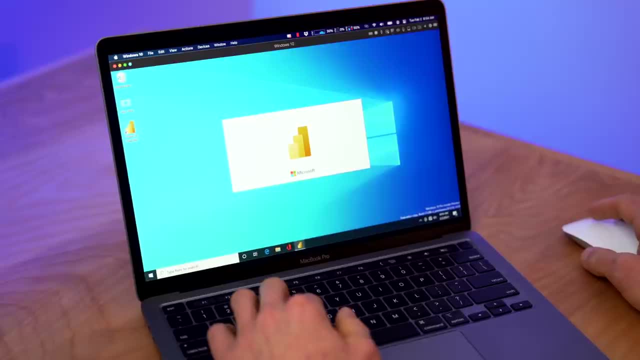 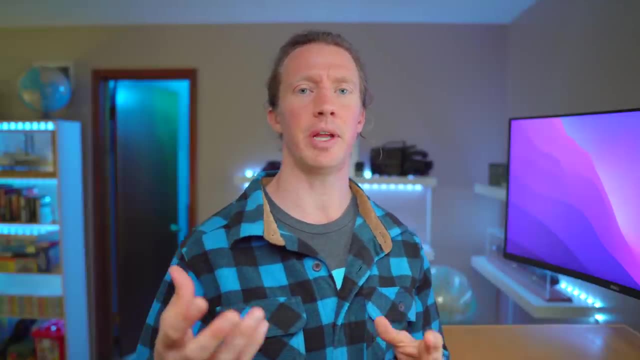 At the time, I was looking to improve my BI tools and an opportunity came up to build a solution using Power BI. As I had a general understanding of this field of procurement, I was able to apply these newly learned skills of Power BI in my role as a procurement analyst, And I was able to apply 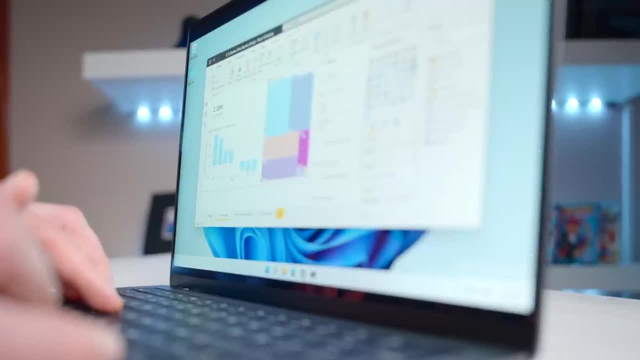 these newly learned skills of Power BI in my role as a procurement analyst And I was able to apply to build this dashboard, But also I was able to actually go more in depth and learn even more about this field of procurement. So for those that are working in an industry or maybe going to, 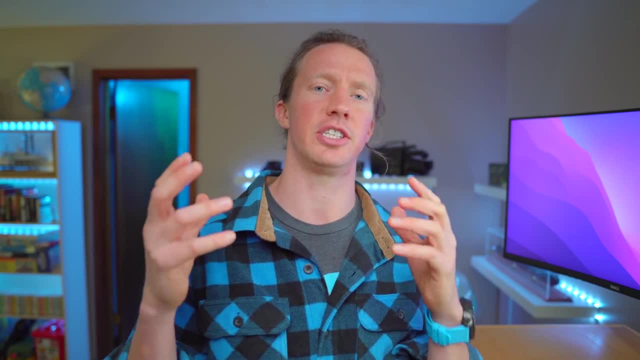 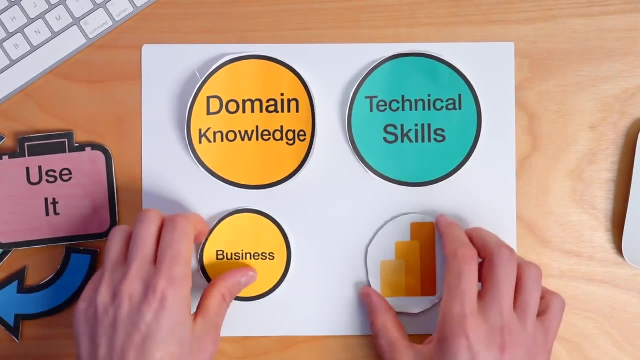 school to learn a certain subject. I highly encourage you to take a similar approach and dive into a tool, while also diving deeper into that domain, so that way you can apply those skills in a relevant project. Last up is soft skills, And this relates to how you work and 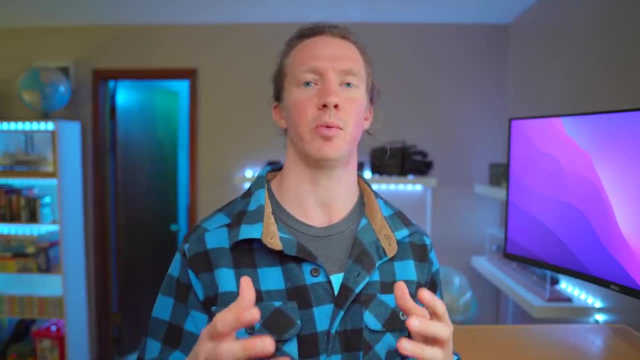 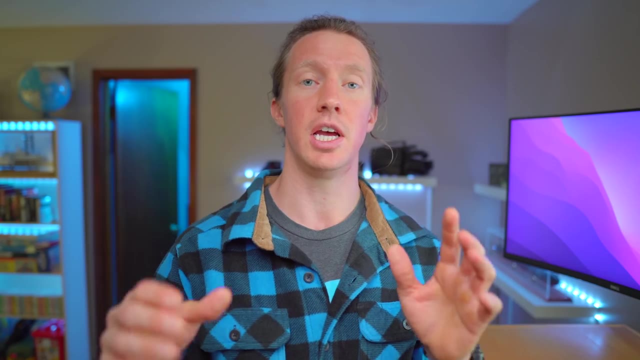 also interact with other people. With the current pandemic, this has shifted the way that we're interacting with each other And instead of doing the normal face-to-face interactions, we've actually shifted this quite differently to using alternate forms of communication. I actually think this is a positive, in that you can actually showcase these alternate. 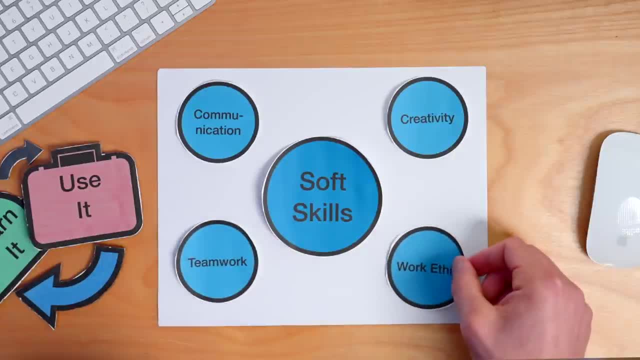 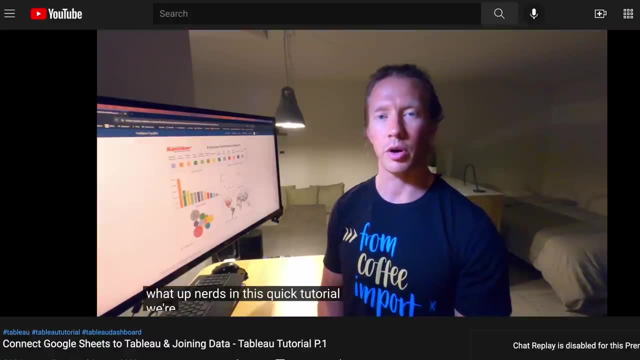 forms of communication in your portfolio and in the projects that you do. So what do I mean by this? Well, when I was learning Tableau, I decided to make a YouTube series documenting my learnings. These videos were not only improving my Tableau skills, but also a way for me to improve my soft. skills of communication. So what do I mean by this? Well, when I was learning Tableau, I decided to make a YouTube series documenting my learnings. So what do I mean by this? Well, when I was learning Tableau, I decided to make a YouTube series documenting my learnings. So what do I mean by? 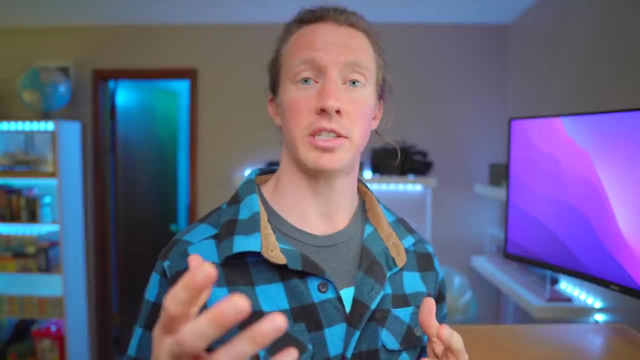 this. Well, when I was learning Tableau, I decided to make a YouTube series documenting my learnings, Where I was getting first-hand feedback on my presentation skills. Now, I'm not saying that you have to make YouTube videos per se. Instead, what I'm saying is that you can use social media. 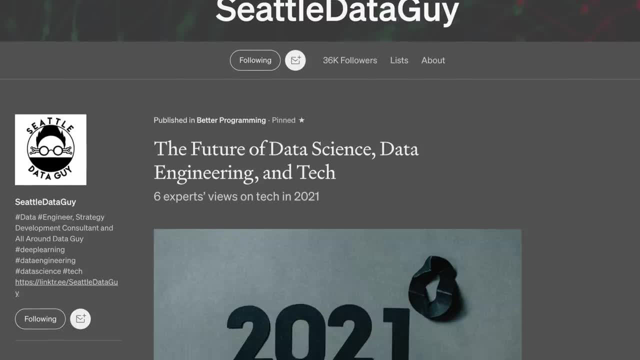 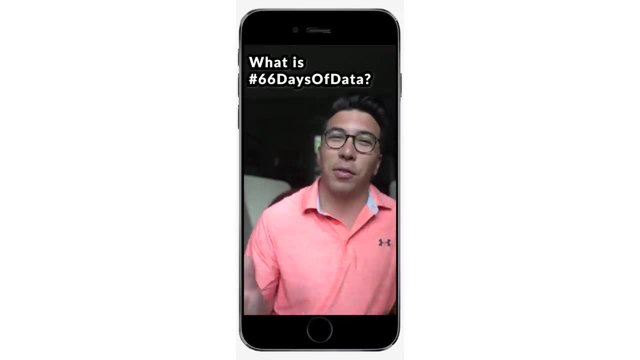 in order to showcase those soft skills that you have, such as writing posts or tutorials on Medium, sharing your code or processes on GitHub or making short form content on Instagram or TikTok. All of these not only have the benefit of working on those technical and soft skills. 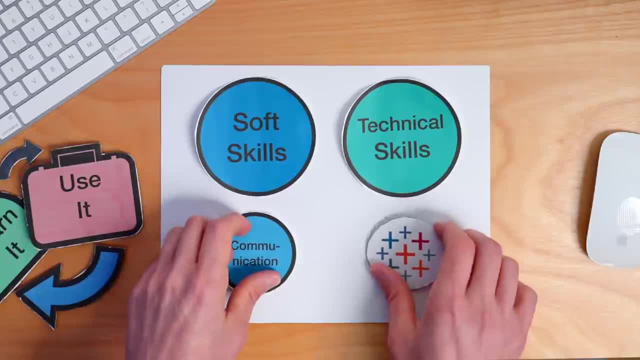 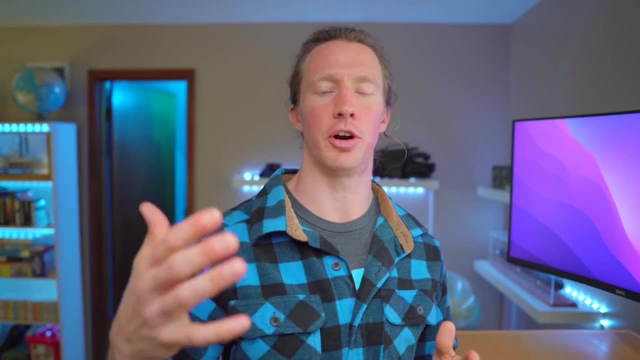 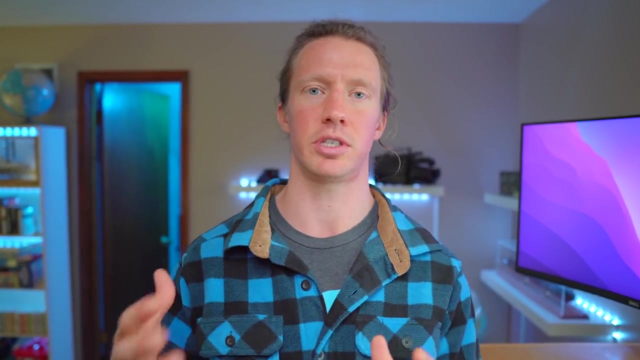 they also are able to be used and showcase your experience for employers to see how you interact with others. All right, so that's my roadmap on how I've learned to become a data analyst. Remember, this is not a comprehensive plan, so you don't need to learn every single skill that I showed here today Instead. 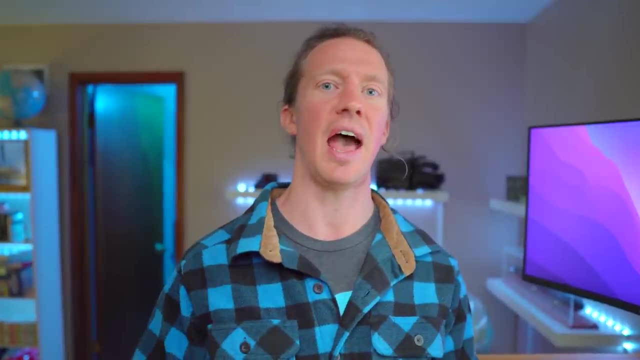 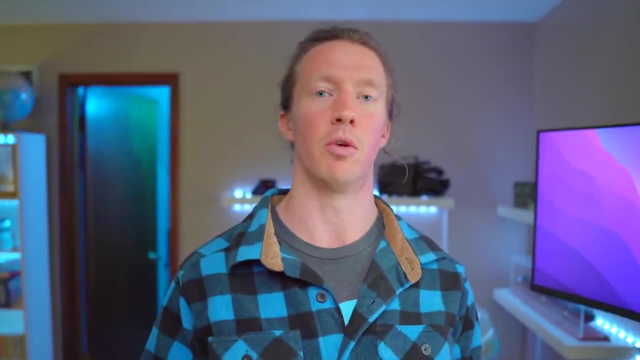 I'd start small right. So start with that one technical skill and add in another skill, maybe analytical or soft skill, that you want to work on, and build a project From there. iterate. Remember: for me, one skill of Excel was good enough to get my first job as an analyst. 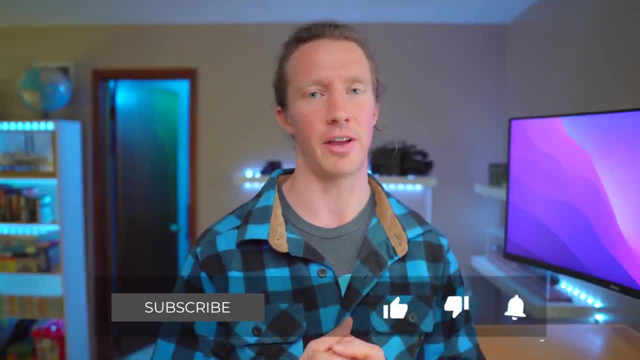 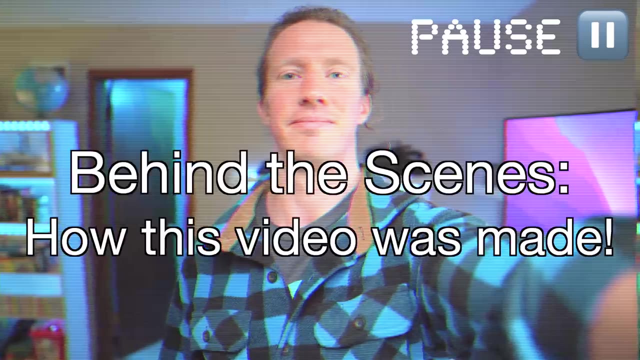 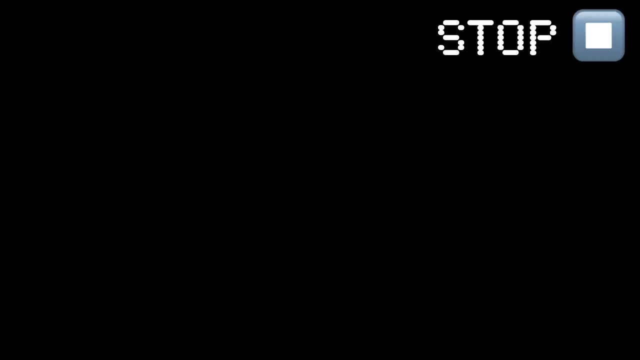 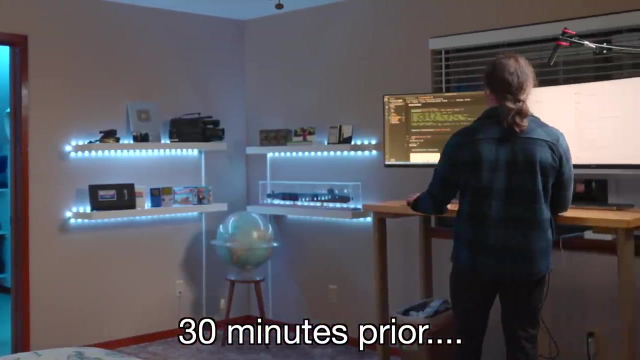 and I feel the same can apply to you as well. As always, if you got value out of this video, smash that like button And with that, we'll see you in the next one. New video from Ken on how to start in data science: Yes. 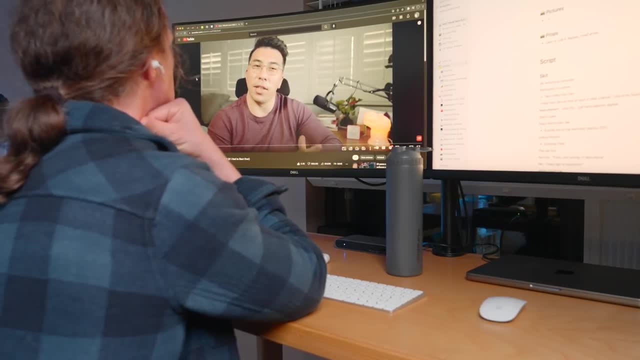 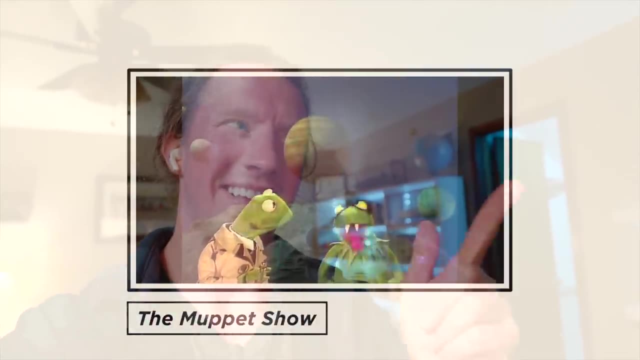 Every year, I like to refresh my advice about how I feel about learning data science from ground zero. The data domain is changing rapidly and as my knowledge grows, I'm going to learn more about data science in the upcoming year. Thank you so much for watching and good luck on your. 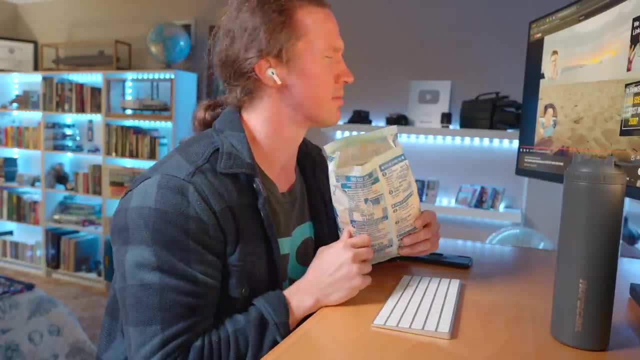 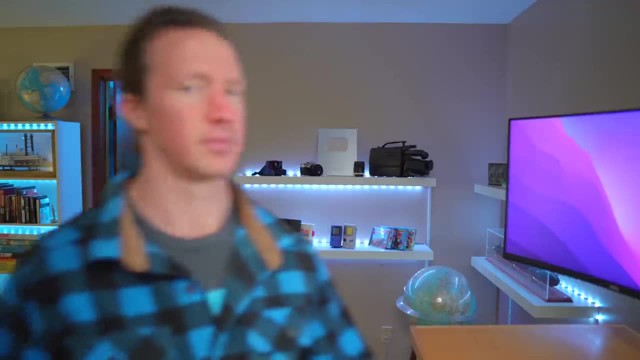 data science journey. Wait a second. we need a video like this, but for data analysts. What up data nerds? I'm Luke, a data analyst, and my channel's on Facebook. I'll see you in the next video.